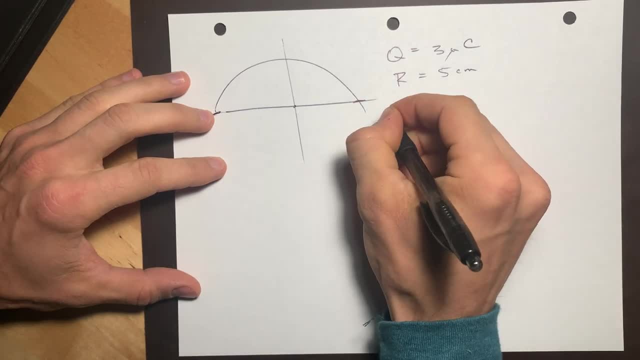 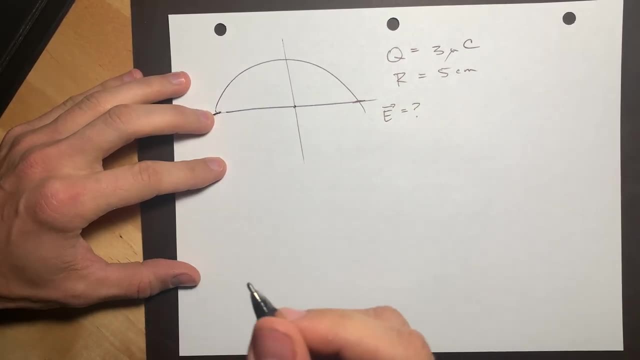 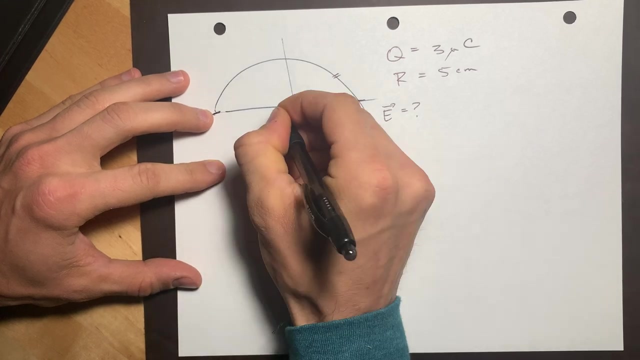 of the ring, What's the acceleration of the electron? But you want to know what's the electric field at the middle here. And so first let's say the electric field is the integral of dE, And then let's say you have some charge here. This is your r hat vector, This is your 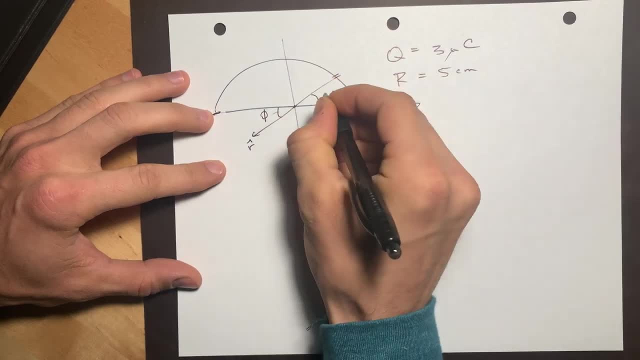 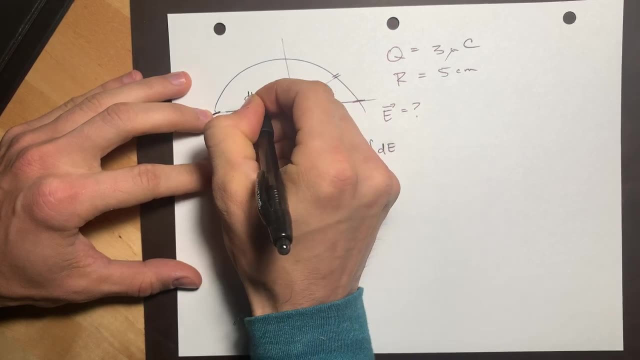 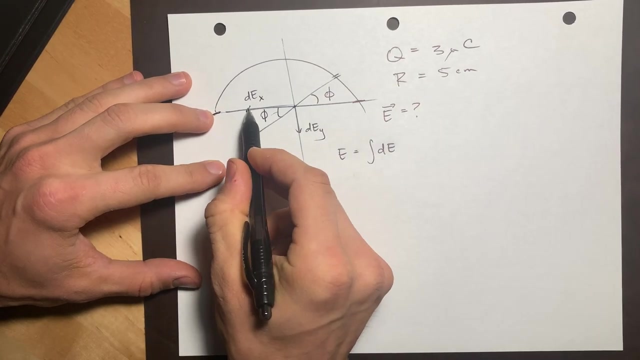 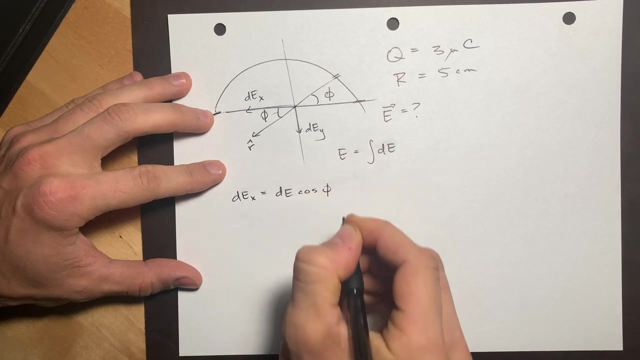 angle in this problem: phi. These are vertical angles. That's the same angle. The component would say: this is dEx and this is dEy, And trig says that this is dEx is equal to dE times cosine phi And dEy is dE sine phi. But it's going in the negative direction. So let's just put a. 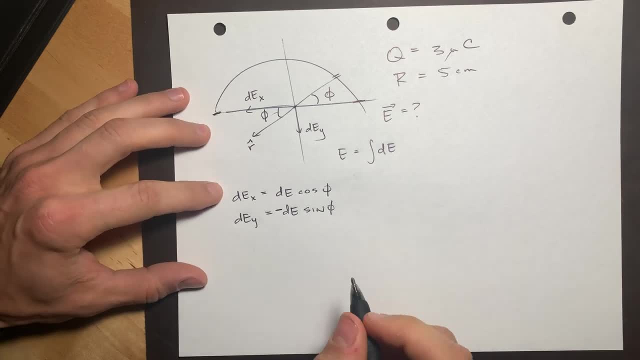 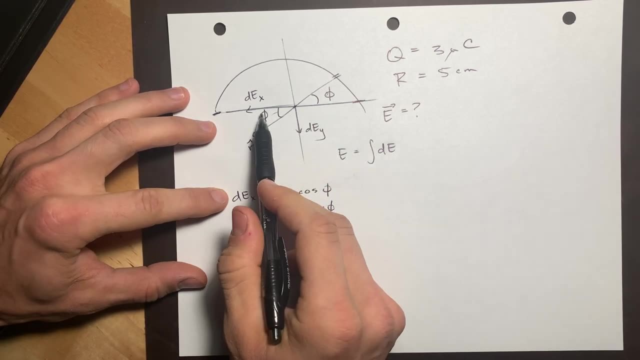 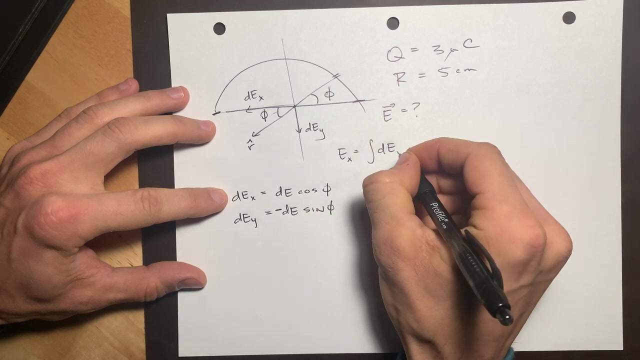 negative sign. in front of that, Now let's just skip ahead and say like if you do the integral of dEx, all the left stuff cancels all the right stuff And this will actually equal zero. So if we do a little x here, 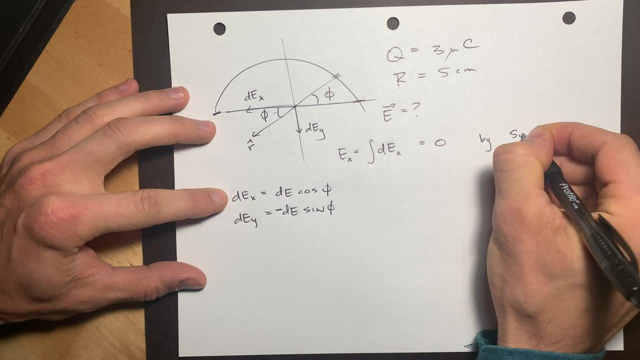 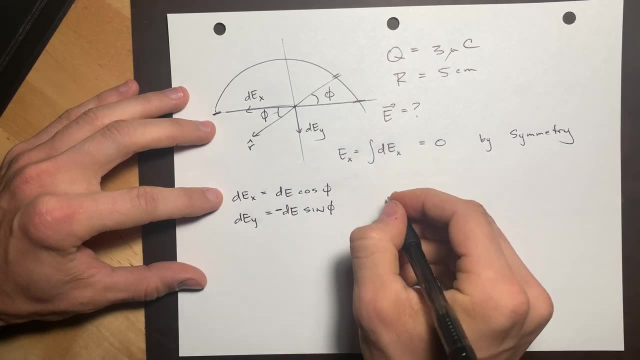 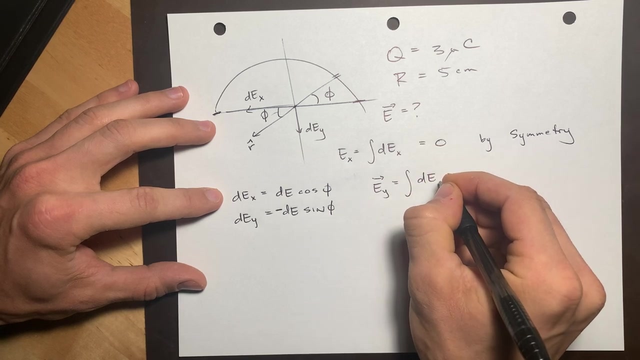 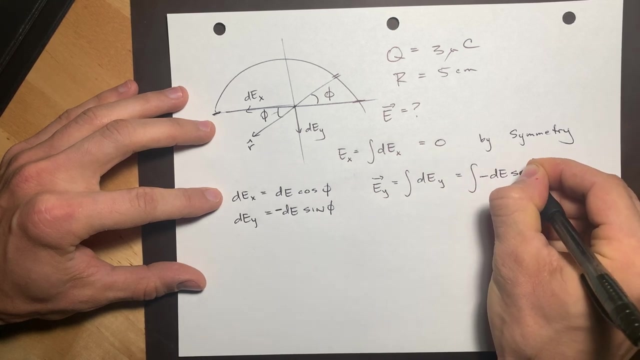 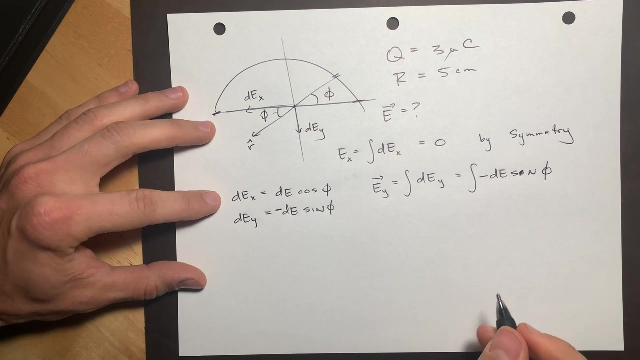 we'd say this would be zero by symmetry. So let's go after the y component. So this is the integral of dEy, which is integral of negative dE. I don't know if I could spell sine phi. So our next task. 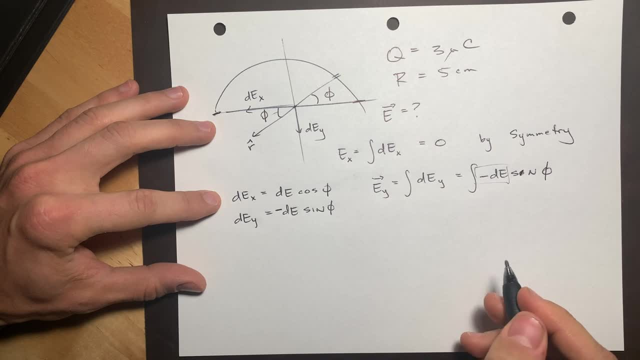 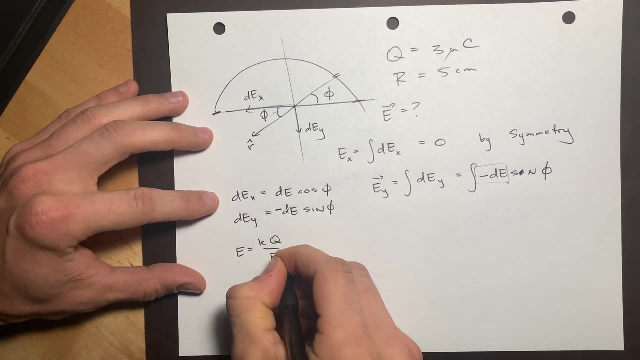 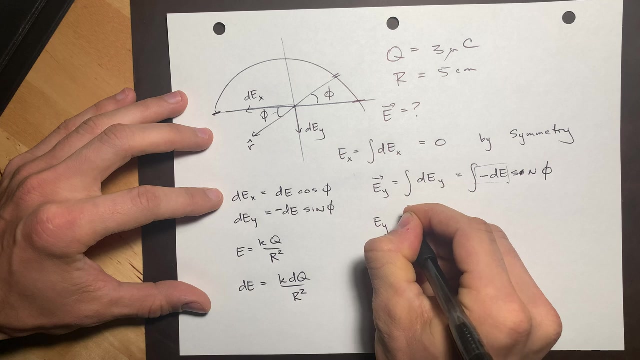 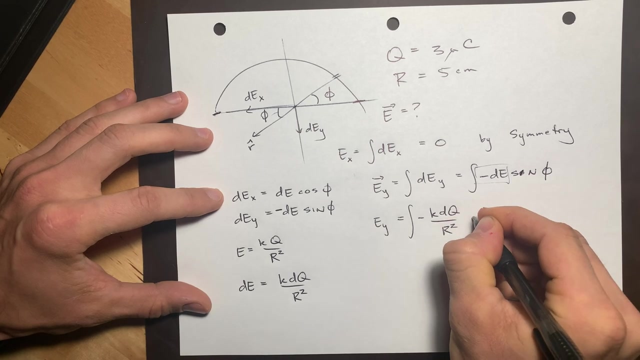 is this guy? What is dE? Well, E is kq over r squared, So dE is kdq over r squared. Okay, we're making some progress. This is the integral of negative kdq over r squared times sine of phi. Now we have to go over dq. We have to try to figure out. 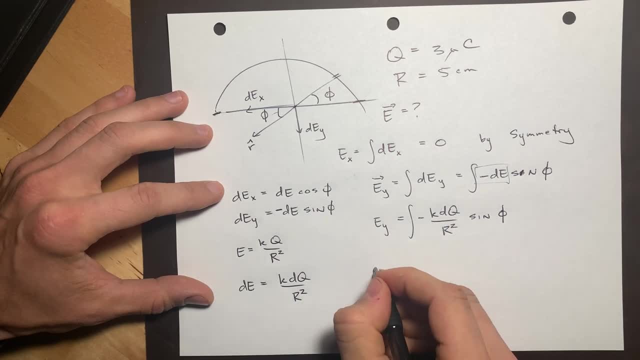 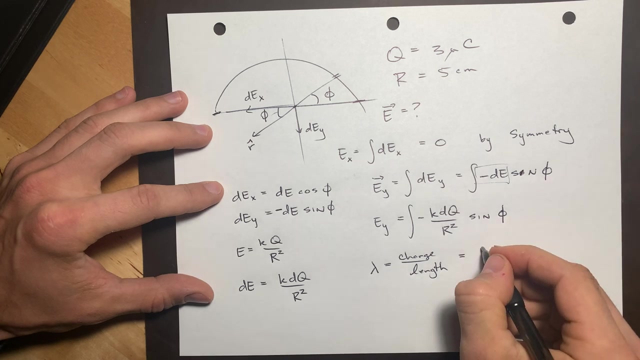 what dq is, And this is a little weird, but we use this letter lambda to be charge per length. This is linear charge density. So this would be, let's say, q over arc length s And let's make it dq over ds. 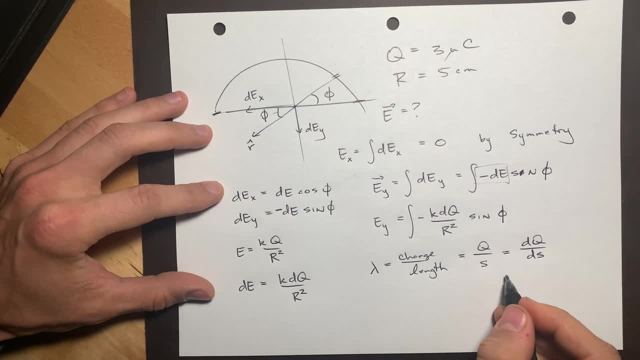 multiply. well, let me think for a second. so yeah, let's multiply over. so we say, lambda, ds equals dq and then realize that ds- I know this is getting into the weeds here- but arc length- equals r times theta. so ds equals r times d theta. 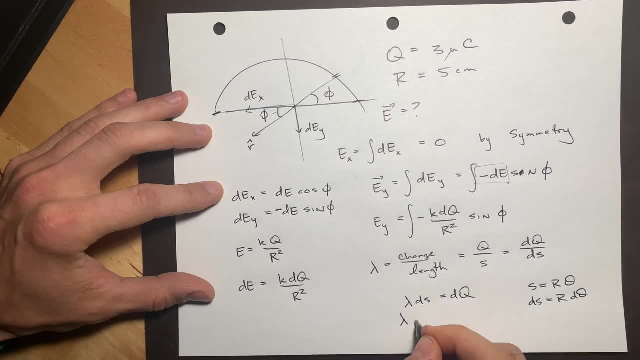 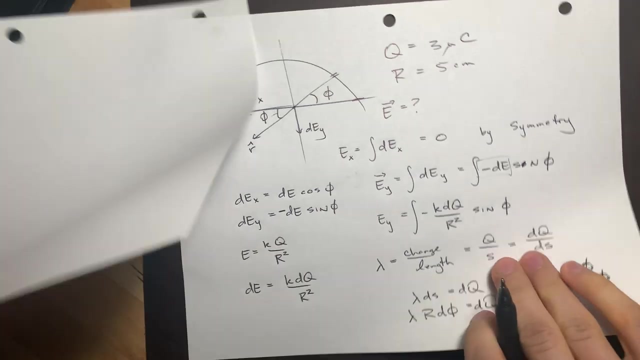 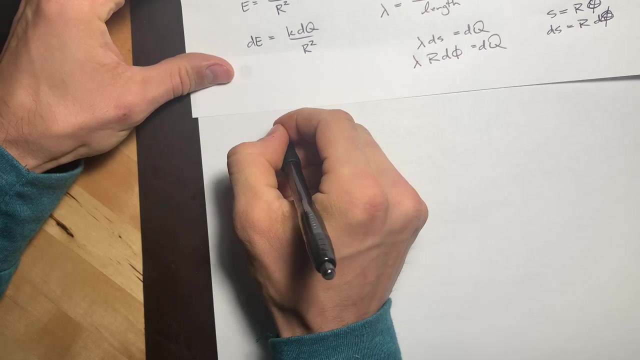 or phi, whatever you want to say. so now, lambda r d phi, just make this a phi to match our earlier angle. equals dq. alright, this is progress. we're almost, we're getting somewhere. so now we'd say that electric field y. 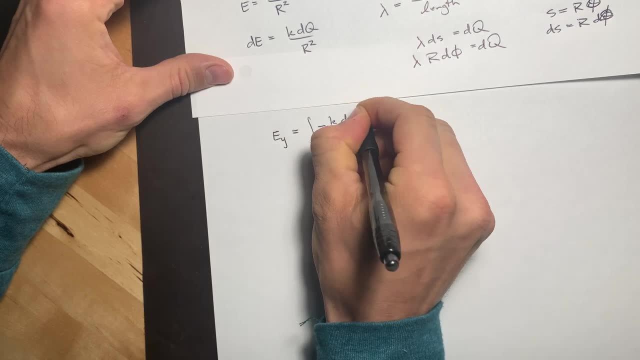 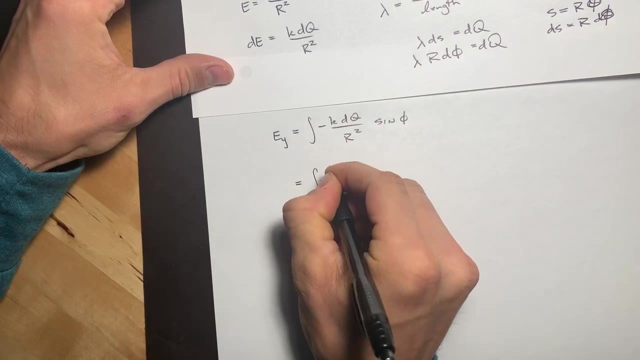 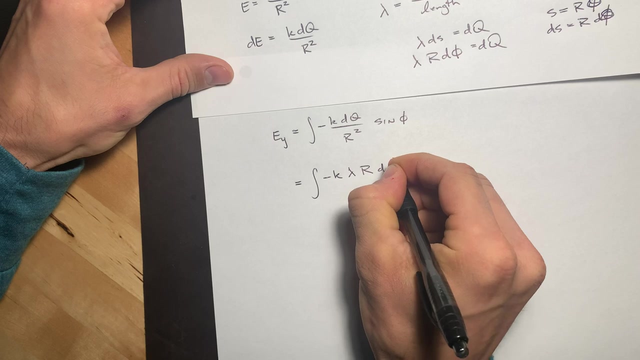 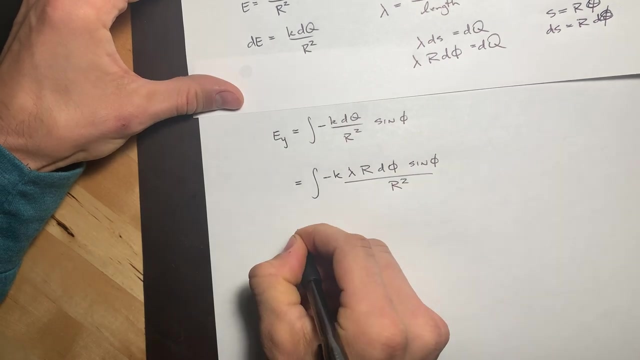 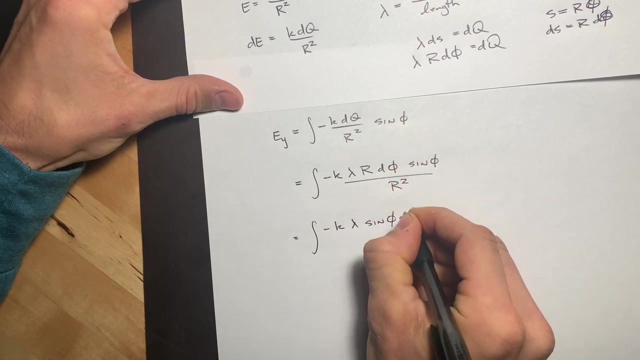 is integral negative k. dq over r squared sine of phi, which is integral negative k. now we're going to replace dq. dq is lambda r d phi and we still have sine phi over r squared, so let's cancel the r. we write it in the normal order. 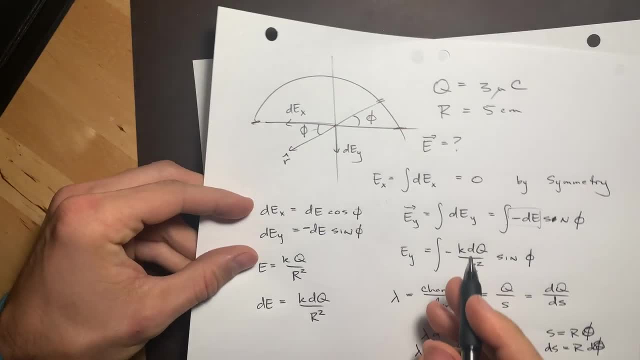 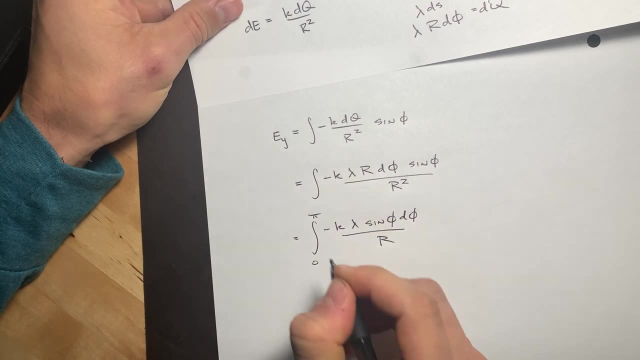 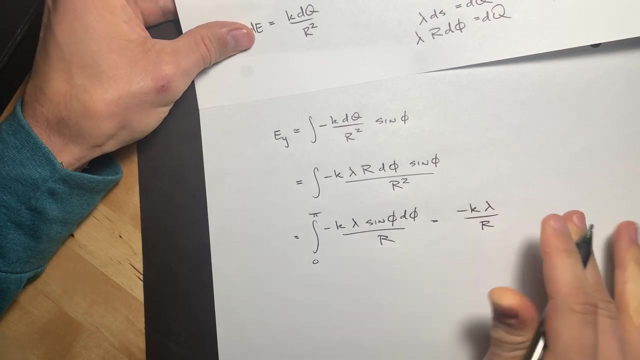 like something like this: now what are we integrating d phi? so in our problem we go from here to here. so what limits are? 0 to pi and we're gonna pull constants to the front. so negative k lambda over r integral from 0 to pi.